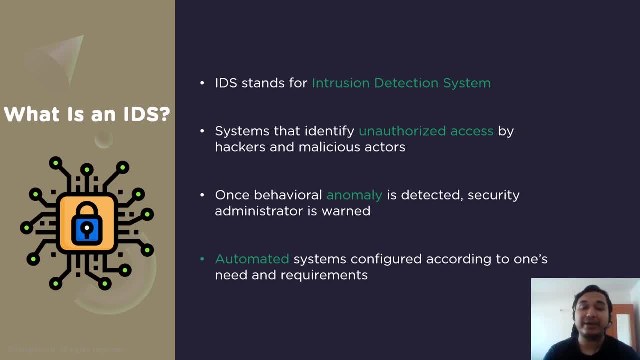 the data carried by network traffic to see if it contains known malware or other malicious content. If it detects this type of threat, it sends an alert to your security team so they can investigate and remediate it. Once your team receives the alert, they must act quickly to prevent an attack from taking. 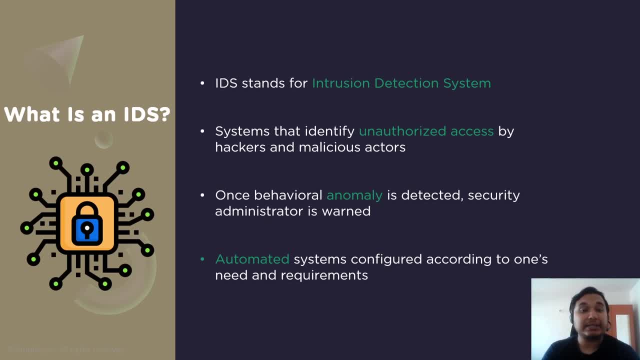 over the system. To ensure that the IDS doesn't slow down network performance, the solutions often use a switched-port analyzer or a text-access port to analyze a copy of the inline data traffic, so that they do not meddle with the actual traffic. However, they do not block. 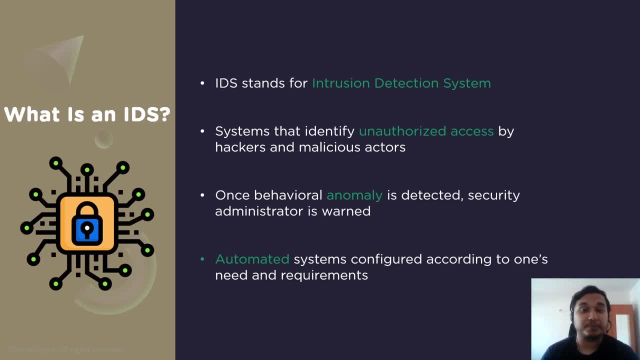 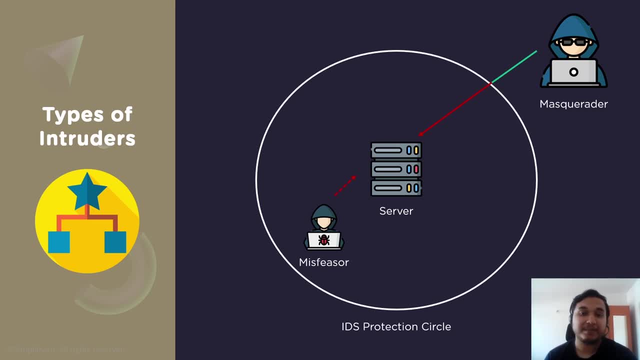 the threat once it enters the network, as intrusion prevention systems do. Regardless of whether you set up a physical device or an IDS program. the system will be able to detect and monitor the threat once it enters the network, as intrusion prevention systems do. Regardless of whether you set up a physical device or an IDS program, the system will be able to detect and monitor the threat once it enters the network, as intrusion prevention systems do. Regardless of whether you set up a physical device or an IDS program, the system will be able to detect and monitor the threat once it enters the network, as. 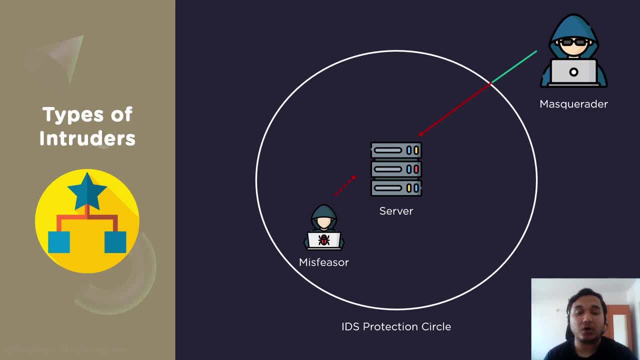 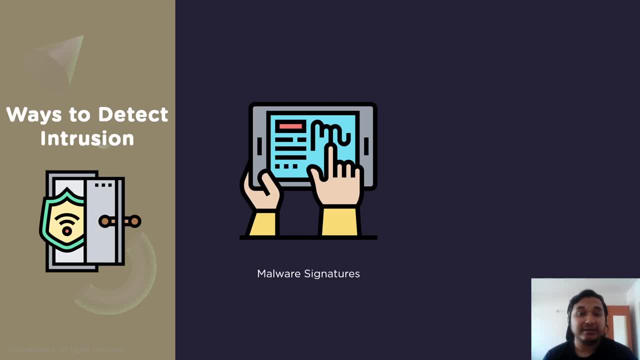 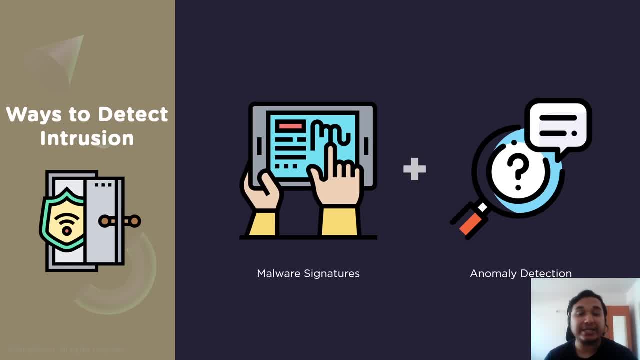 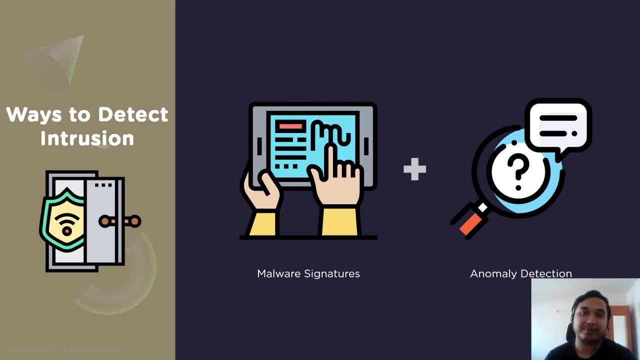 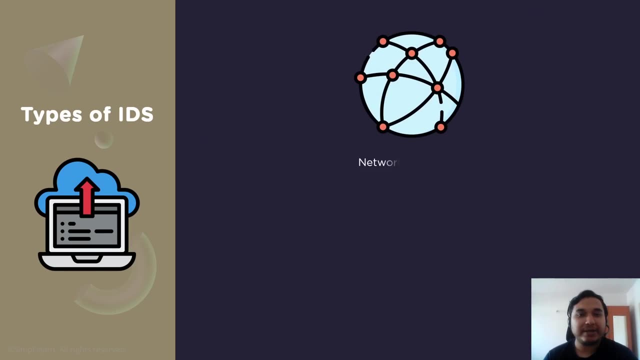 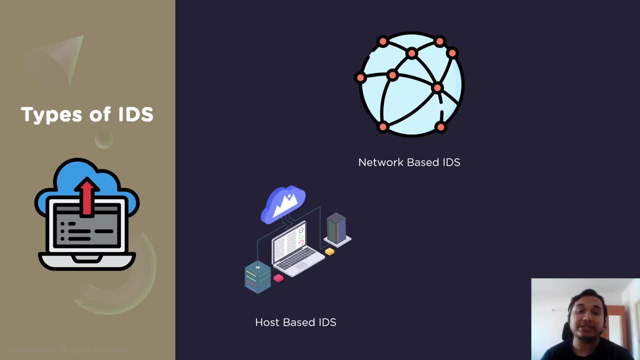 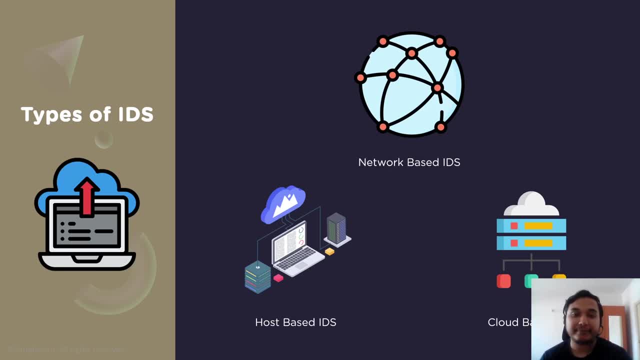 the threat once it enters the network, as intrusion prevention systems do. Regardless of whether you set up a physical device or an IDS program. the system will be able to detect and monitor the threat once it enters the network, as intrusion prevention systems do. Regardless of whether you set up a physical device or an IDS program, the system will be able to detect and monitor the threat once it enters the network, as intrusion prevention systems do. Regardless of whether you set up a physical device or an IDS program, the system will be able to detect and monitor the threat once it enters the network, as. 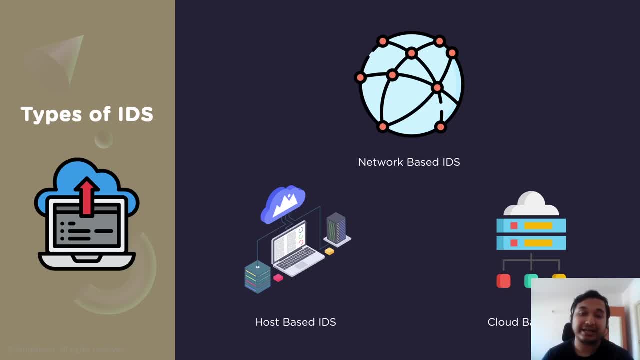 intrusion prevention systems do, Regardless of whether you set up a physical device or an IDS program. the system will be able to detect and monitor the threat once it enters the network, as intrusion prevention systems do, Regardless of whether you set up a physical device or an IDS program. the system will be able to detect and monitor the threat once. 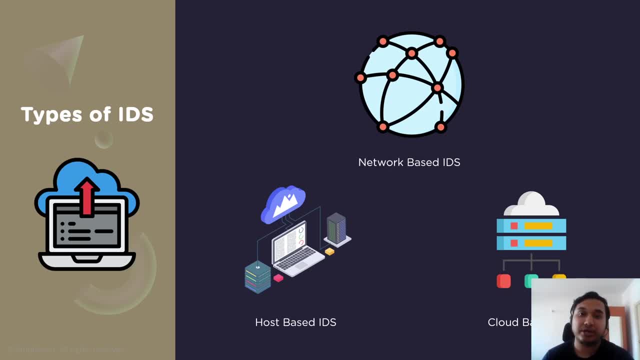 it enters the network, as intrusion prevention systems do, Regardless of whether you set up a physical device or an IDS program. the system will be able to detect and monitor the threat once it enters the network, as intrusion prevention systems do. Regardless of whether you set up a physical device or an IDS program, the system will be able to. detect and monitor the threat once it enters the network, as intrusion prevention systems do. Regardless of whether you set up a physical device or an IDS program, the system will be able to detect and monitor the threat once it enters the network as intrusion prevention. systems do, Regardless of whether you set up a physical device or an IDS program. the system will be able to detect and monitor the threat once it enters the network, as intrusion prevention systems do, Regardless of whether you set up a physical device or an IDS program. 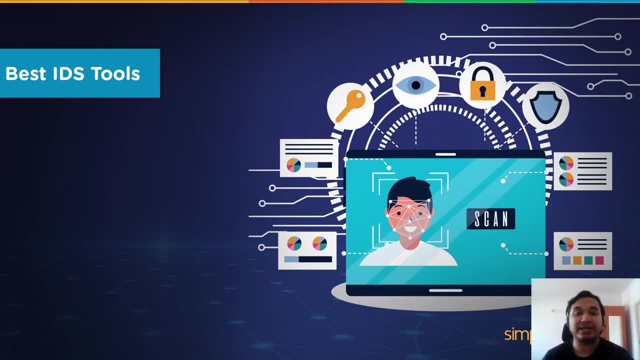 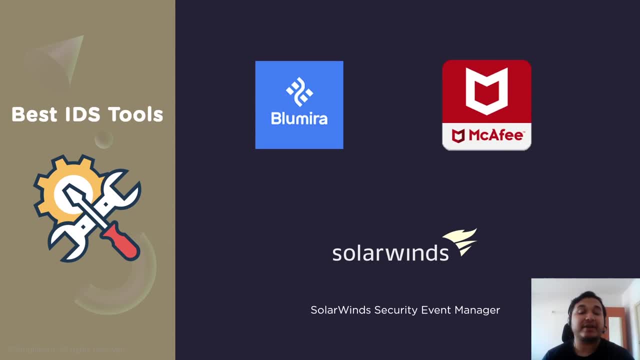 the system will be able to detect and monitor the threat once it enters the network, as intrusion prevention systems do. Regardless of whether you set up a physical device or system and a host-based IDS system, The solution can let you discover all kinds of malicious attacks and help you protect. 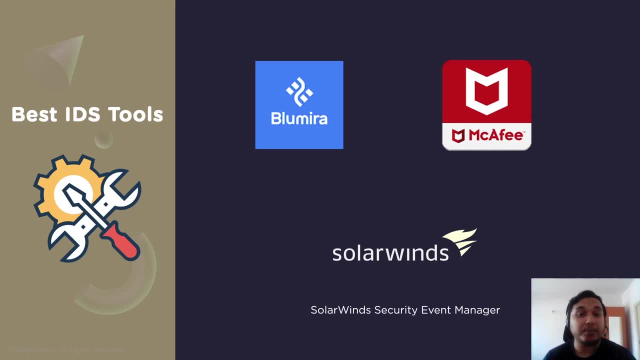 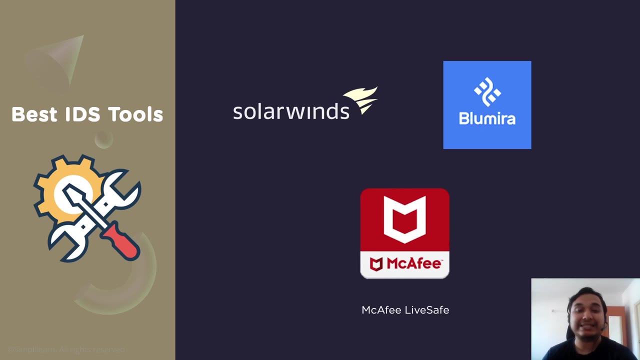 your network from harm. It is also designed to enact both signature-based and anomaly-based intrusion detection by comparing sequences of network traffic against a set of customizable rules. Next we have the McAfee LiveSafe. McAfee- LiveSafe is an intrusion detection system designed to bring real-time threat. 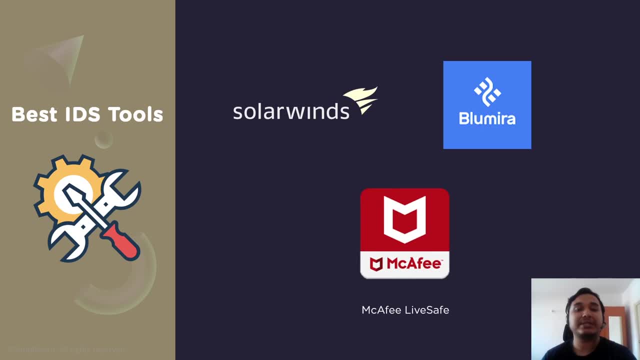 awareness to your physical and virtual networks. It uses signature-based intrusion prevention and anomaly-based intrusion detection, along with emulation techniques, to spot and identify malicious activity. McAfee is also built to correlate threat activity with application usage, which can further prevent network issues stemming from cyber attacks. 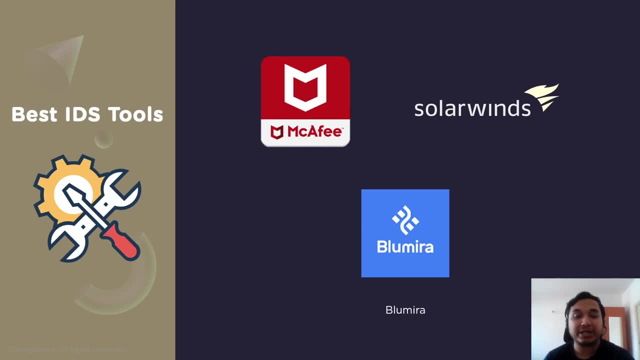 Next we have Blumera. Blumera is a security information and event management platform built to enact threat detection and responses across your cloud and on-premises environments. It is designed to continue threat detection across your cloud and on-premises environments. 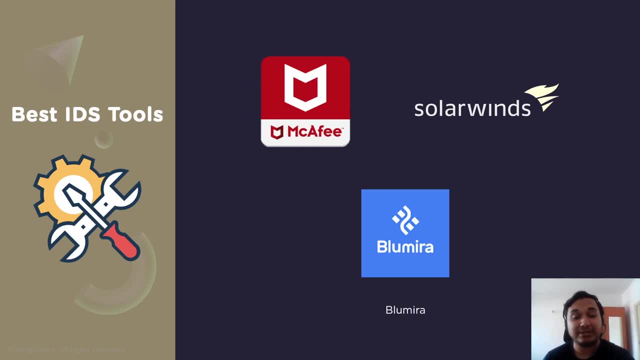 It also enjoys multi- gabby system and is able to remotely monitor your IT infrastructure for suspicious activity and misconfigurations, both of which could result in data leaks and compliance breaches. It enables you to respond to an attack in progress and stop malicious acts in their 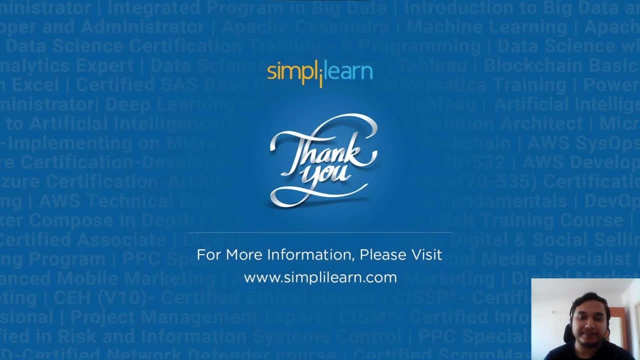 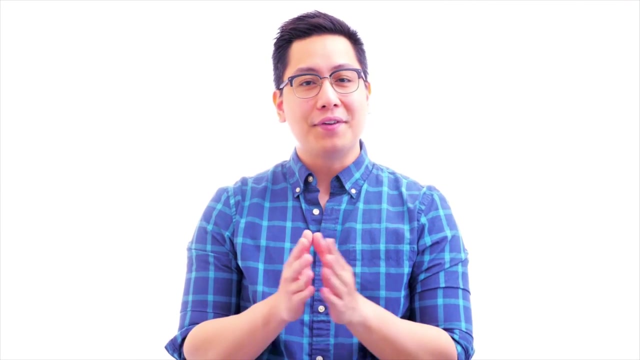 tracks. Hope you learned something new today. Please let us know if you find any issues regarding ideas in the comments section below. Subscribe to our channel for more videos like this. Thank you for watching ィ. If you like this video, subscribe to the SimplyLearn YouTube channel and click here to watch similar. videos To nerd up and get certified: click here.